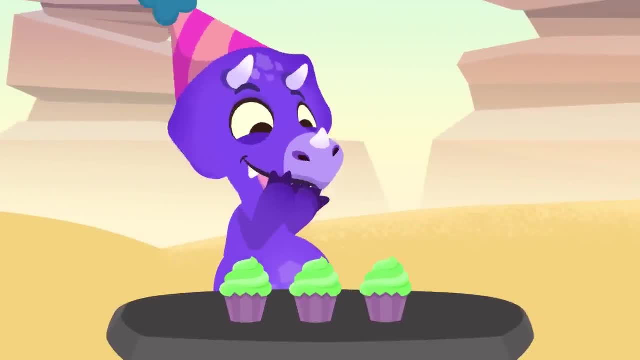 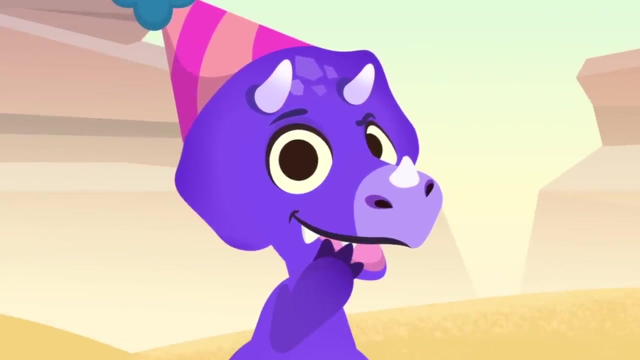 Whoa, These cupcakes look awesome. Sari, What is it? Are you hungry? Come on, don't be shy, Have one In one bite. You're never full. Sari, Do you know? you've just done a subtraction without realizing it. 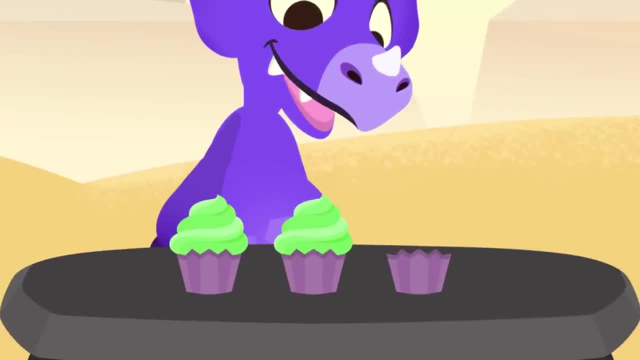 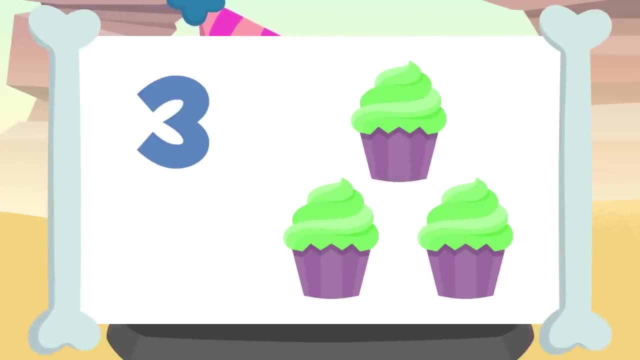 We subtract to know how many things we have left after taking away some of them, just like you did with these cupcakes. For example, before there were three cupcakes on the table and you've eaten one. So if we take one away from three, there will be one and two cupcakes left. 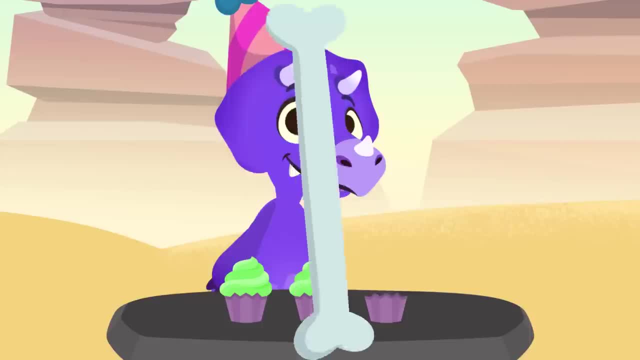 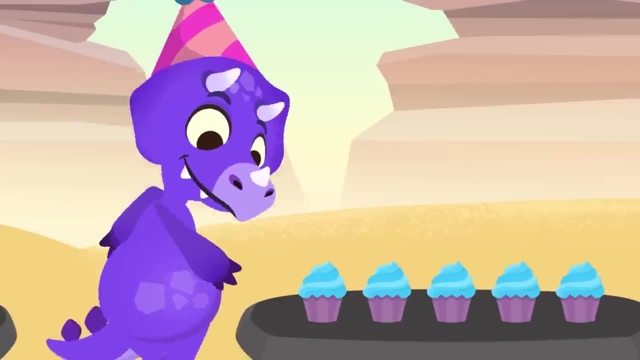 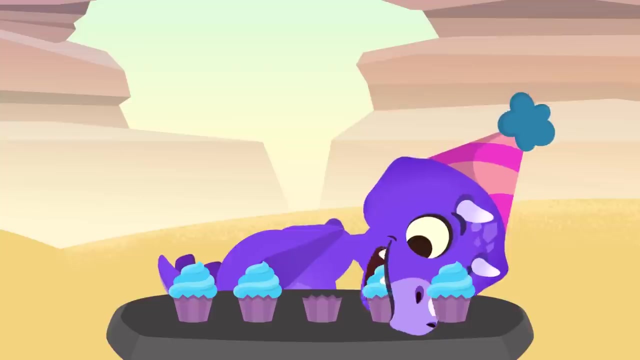 Three minus one equals two. Well done, We have done our first subtraction. See how easy it was. Yum yum, These cupcakes are mouth-watering. But wait, Sari, You've subtracted again without realizing How many are there left? 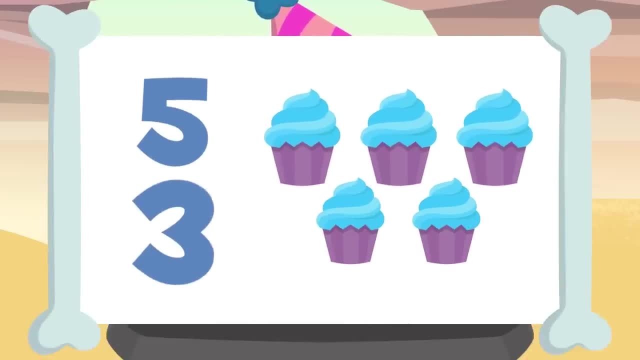 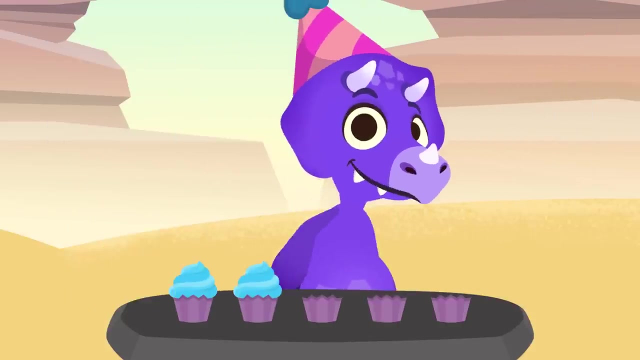 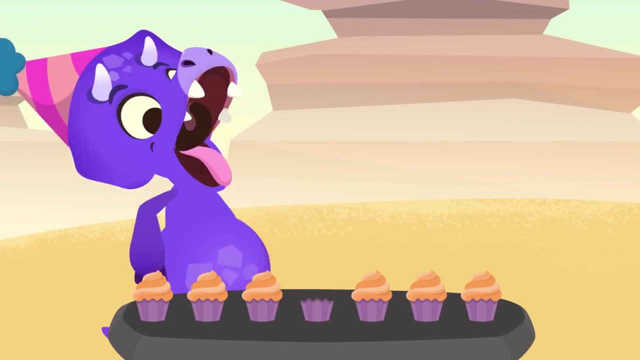 This time there were five cupcakes and you've eaten three. So if we take away three from five, there will be one and two cupcakes left. Two, Five minus three equals two. Awesome, Are you still hungry? There's nothing we can do with you. Sari, is there? 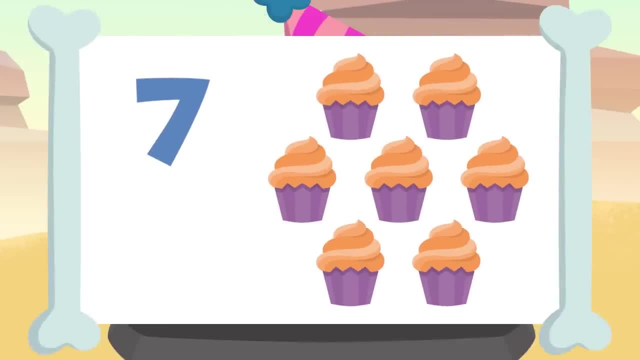 On the table. there were six cupcakes- Awesome, Are you still hungry? There are seven cupcakes and you've eaten four of them. If we take away four from seven, one, two, three and four, the result is one, two and three. 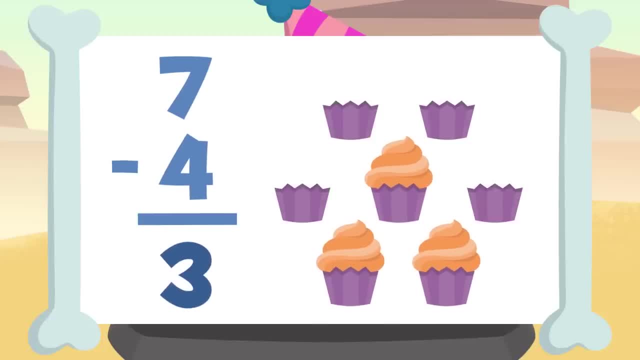 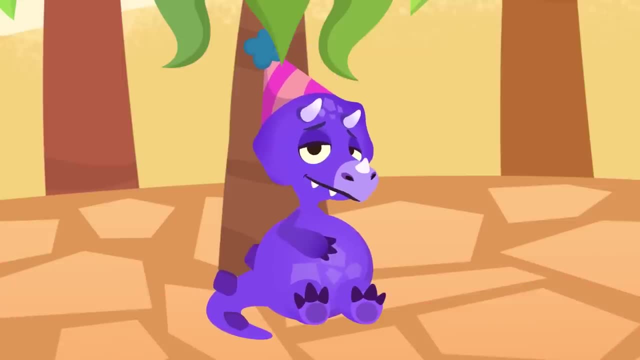 Three Seven minus four equals three. Good job, Sari. Do you like subtracting? I told you, Sari, there were too many cupcakes. Well, let's recap the subtractions we practiced today. All right, We can also do horizontal subtractions. 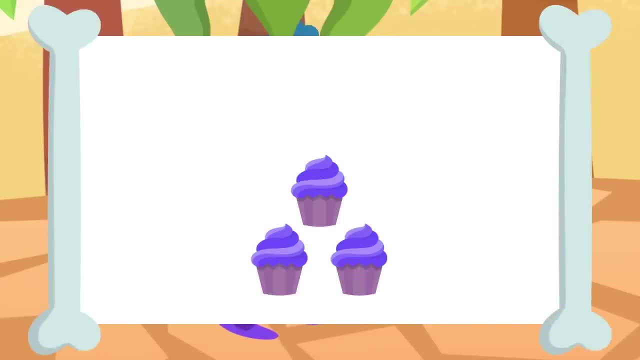 It's done in the same way. Pay attention: Three minus one equals one and two. Three minus one equals two. Awesome, Let's do the next one. If I take away the three cupcakes from these five cupcakes- one, two and three.